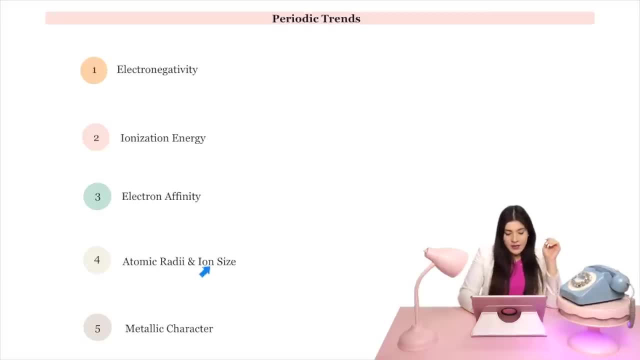 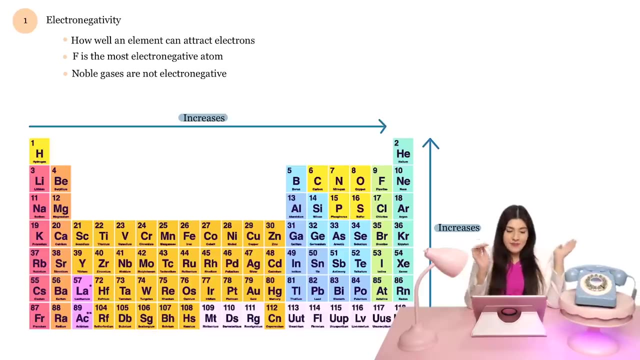 and then I included technically a sixth one, but let's just start off with electronegativity. okay, So starting off with electronegativity, what is it? Electronegativity is telling us how well an element can attract electrons, right? 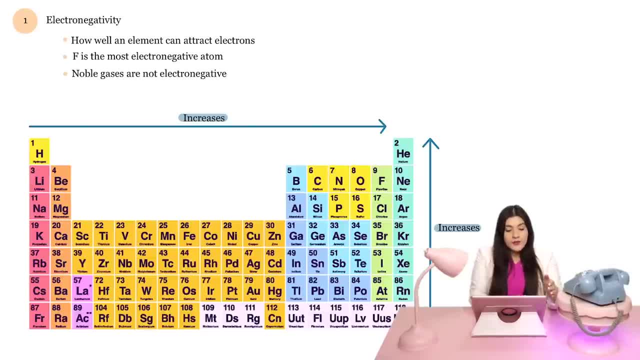 The trend for electronegativity is going to increase as we move across the periodic table and then as we move up a column. So really, what I want you to think of is that fluorine is the most electronegative atom And then- this is something to note- that your halogens typically are the highest in electronegativity. 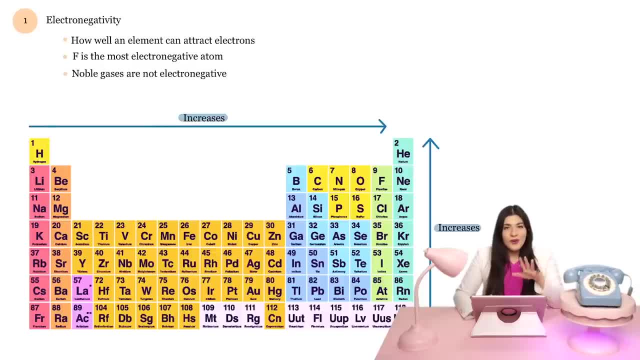 And there is something to also know. There's an exception here where noble gases are not electronegative whatsoever, though they seem like they'd fit the trend here where, okay, it's telling us, yeah, those would be the noble gases would be the highest in electronegativity. But in this case it's not. Instead, noble gases have eight valence electrons, meaning they're happy. They don't want to attract any more electrons because they have enough. That's why the halogens are the best, Because they have seven valence electrons and they want to attract another electron to complete. you know that octet or have eight valence electrons. 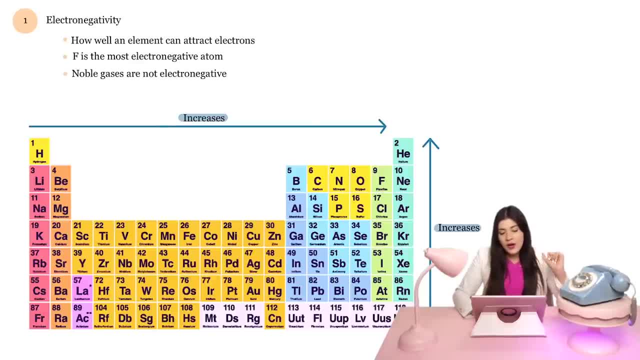 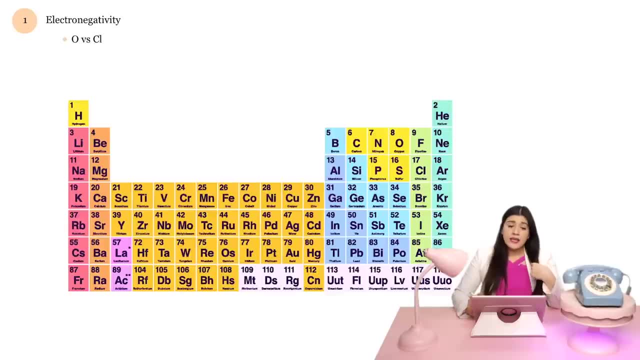 So fluorine is going to be the easiest way to understand and just instantly remember: whatever is closest to fluorine is going to be more electronegative. Now let's do an example. Okay, so this is a common case where let's say, if you're given, which atom is the most electronegative? 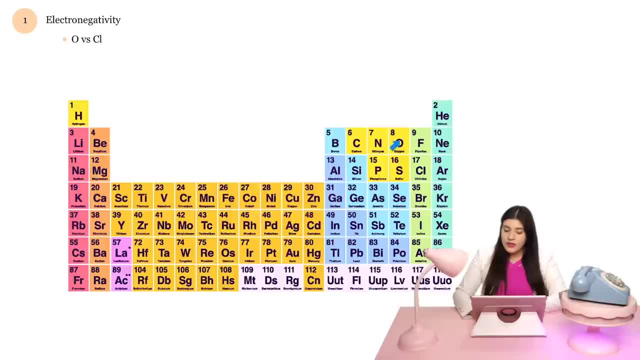 Is it oxygen or is it chlorine, And this one's a little bit difficult to tell. So, looking at the trend, well, they're really close to fluorine. They're both right there with fluorine, right? I'd say they're equidistant to each other. 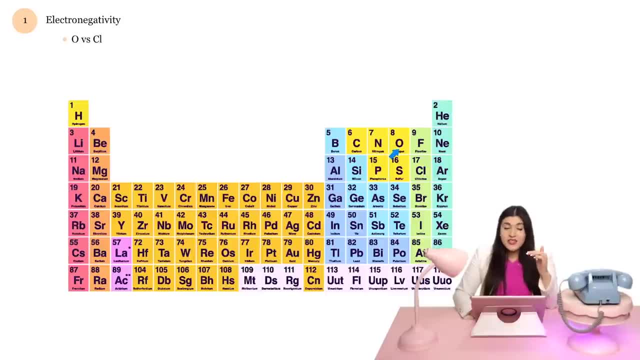 But in this case, the one that is higher up is actually going to be the most electronegative. So that's going to be your tiebreaker. If you're not too sure which one is going to be more electronegative, then it's the one that is higher up on the row, or, you know, on the same row as fluorine. 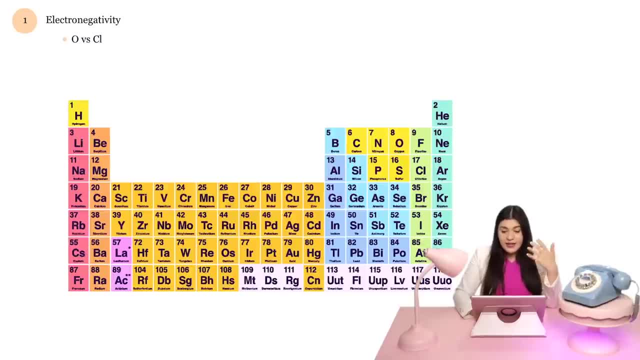 That's going to be more electronegative. Now, if we had something like, let's say, nitrogen and chlorine, those are not the same distance away from fluorine, So chlorine would have been more electronegative in that case. 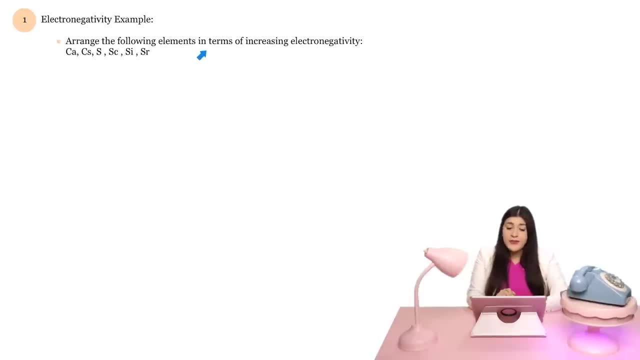 Let's do an example. So this question is asking us to arrange the following elements in terms of increasing electronegativity. So we're given all of these different elements Whenever it's telling us increasing order. what we're essentially looking at is we're looking at the lowest to the highest. 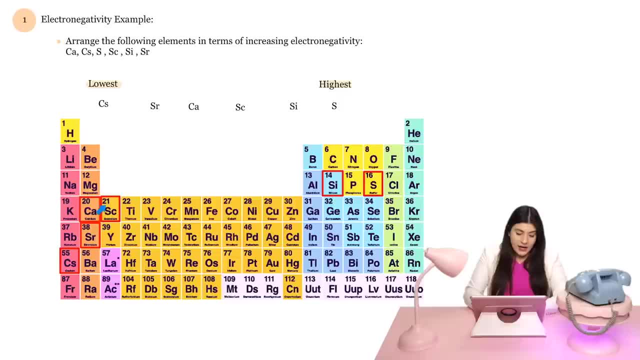 And what I'm going to do is I'm going to identify Where everything is. I went ahead and just boxed in red where every single element that we're asked to order place an order is. So whatever is closest to fluorine is going to be the highest. 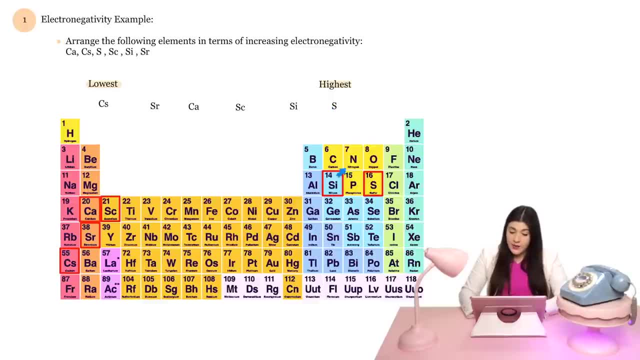 That's why sulfur is the highest, Following that is going to be silicon, And then the next one is right here, Because, remember, anything that's closest to fluorine is going to be the most electronegative. Now that these, we know, are not electronegative, what we're essentially looking at is the ones that are higher up and more towards the right. 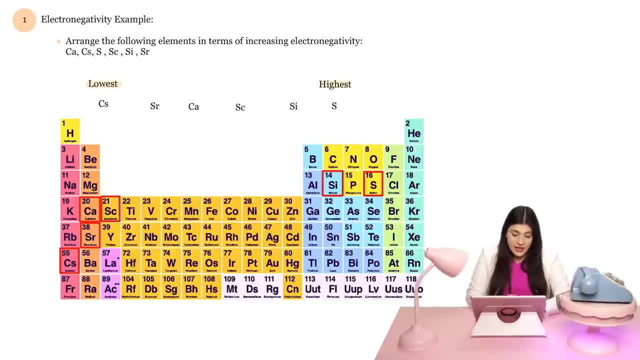 Of the periodic table, Then those are going to be more electronegative. So that's why we have SE, That's why we have CA. That's next. This is a little bit below. So SR. And then CS is the very, very lowest in electronegativity, since it's the furthest away from fluorine. 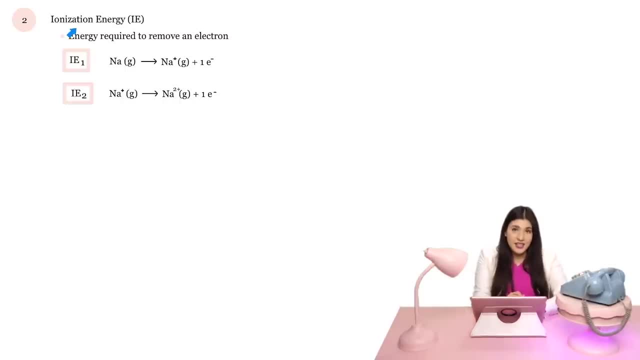 The next type of periodic trend that we'll go over is ionization energy, And sometimes you'll see this abbreviated as IE. Now, what ionization energy is? it's the energy required to remove an electron, And specifically we're looking at these atoms in their gas state. 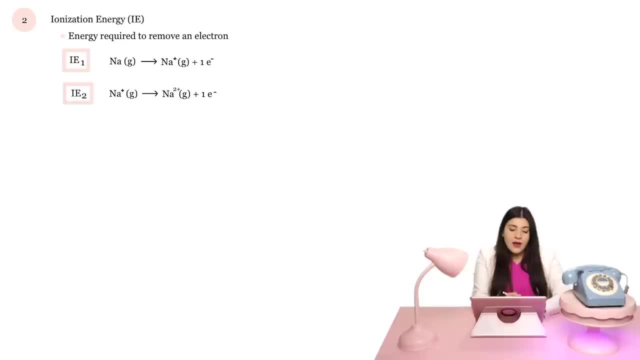 So you'll notice that some of these atoms are going to have more than one ionization energy. Some could have one, two, three and so on. Let's say, if we're looking at this example here, at sodium, where this is in its gas state and it's neutral. 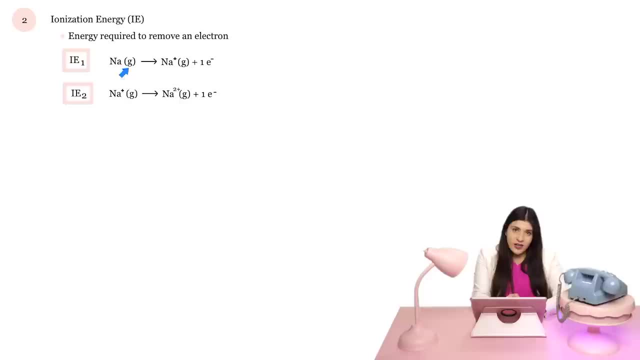 There is no charge whatsoever If I'm trying to remove an electron. remember, electrons are negatively charged. So if I remove an electron, this now becomes positively charged, right, Because I removed something. So if I remove something negative now, this is a cation or a positive charge. 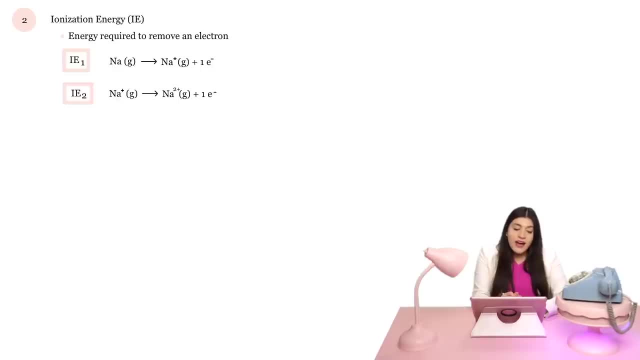 So this is a positive charge, And then I of course have to have the charges be the same. So, since this is neutral and this is a plus one and this is a negative one, those would cancel each other out, making the charge be balanced on both sides. 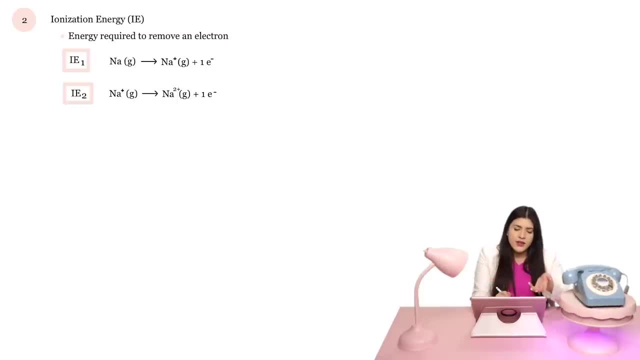 which we have to have, since this is a balanced reaction. So this just tells me: I'm removing one electron so far, And just note that you have to. You have to just remove one electron at a time. You can't. You can't remove two electrons or three electrons at a time. 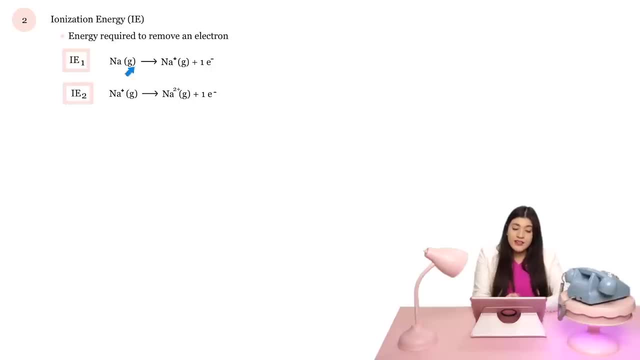 It's only one by one. So this is our first ionization energy. If I were to do this again, then I would take this Na plus and then I would remove another electron. So now this is a two plus charge, And I again show that this is one electron being removed. 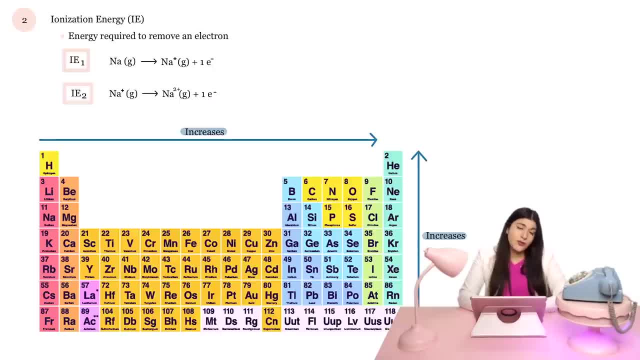 The trend for this is really similar to our electron negativity that we did before. The same way, it's going to increase, the exact same way that we saw before, And this- this is specifically describing the ionization energy of our first ionization energy. 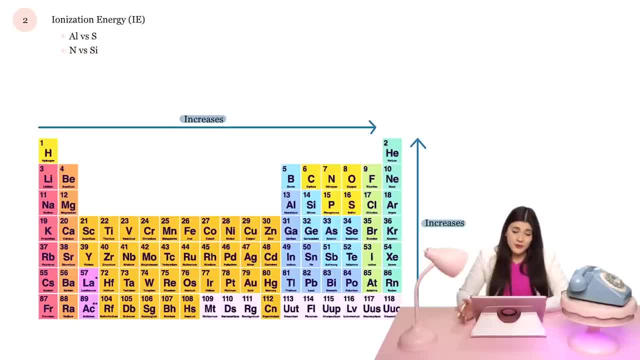 which is the most common one that you will see. Let's do an example. So let's do both of these. If I were to compare aluminum and sulfur, and I'm trying to see which one has the highest ionization energy based on this trend, 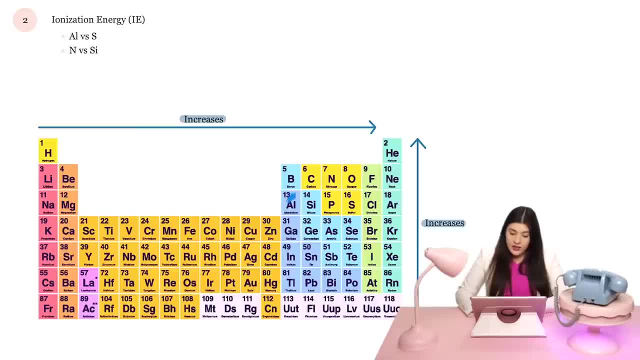 So sulfur is here, And then aluminum is right here. So which one is, Once again, closest to fluorine? Well, that's going to be sulfur. So I know sulfur is going to be the one that has a higher ionization energy. 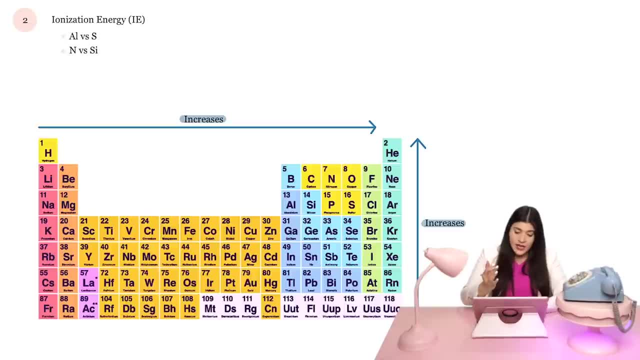 And if I were to look at, let's say, nitrogen versus silicon, let's identify where that is on the periodic table: Here's nitrogen, Here's silicon. Well, nitrogen is higher up And I know that, since that's higher up and it's a little bit closer to fluorine. 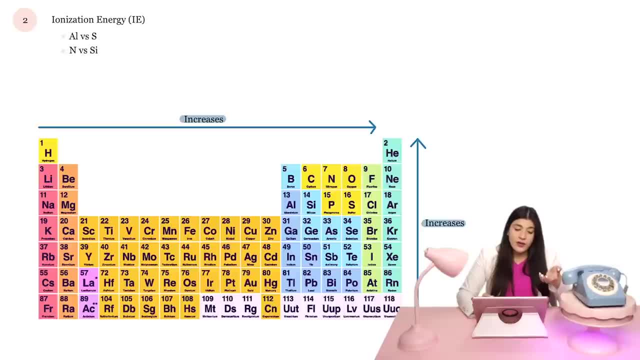 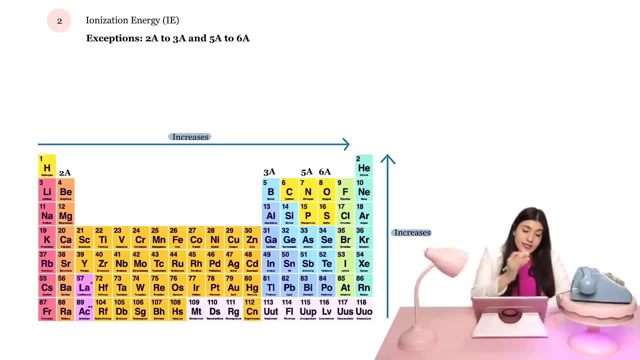 that's going to be also the one that's larger. It has a larger amount of ionization energy. So that's going to be. Those are my answers in this case. Okay, So let's say, if I were to try to now compare two atoms or elements that are the same distance away from each other, 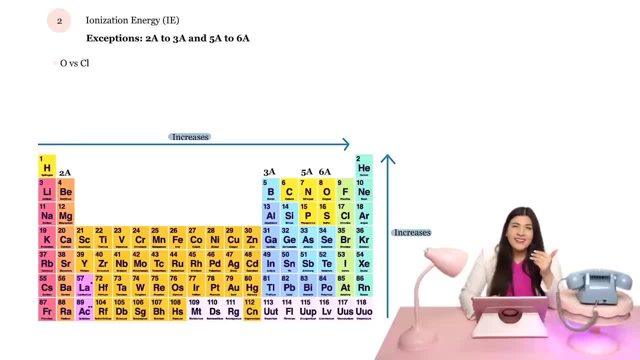 Well, instead of choosing the one that's higher up, that doesn't apply in this case. So for electronegativity that worked. The one that was higher up was the more electronegative atom, But in this case it's not possible to actually tell. 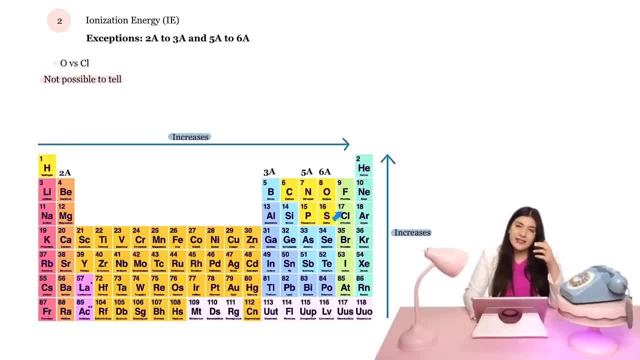 Okay, So if they are the same exact distance from each other, then unfortunately it's just. It cannot be determined which one has a higher ionization energy. Now there's another exception here, where Note that I actually put what each column is on the periodic table, the ones that have exceptions. 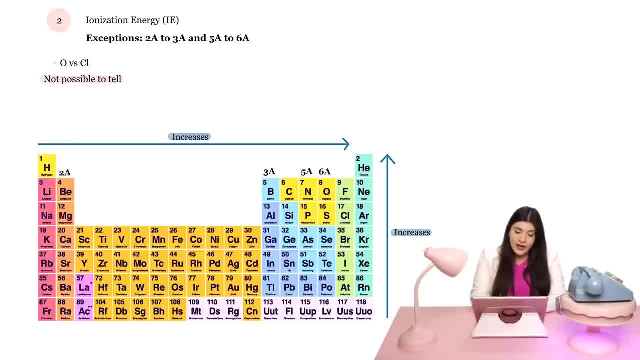 If we were looking at and comparing elements from 2A and 3A. there's an exception there. Let's say, if I were comparing, And actually this is 5A to 6A, but let me go to There, we go. 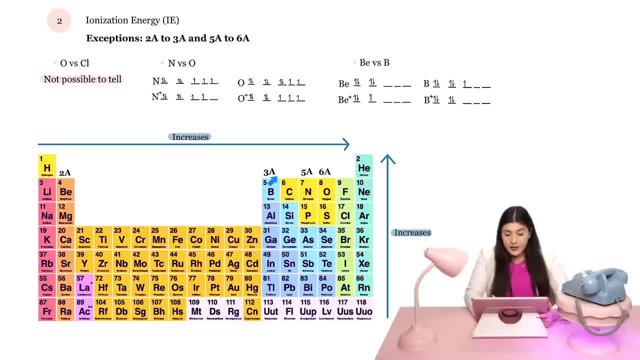 Okay, This one. So if I were going from 2A to 3A, so beryllium to boron, and let's say I wanted to remove an electron, Well, here I brought in the energy diagrams and this is going over electron configuration. 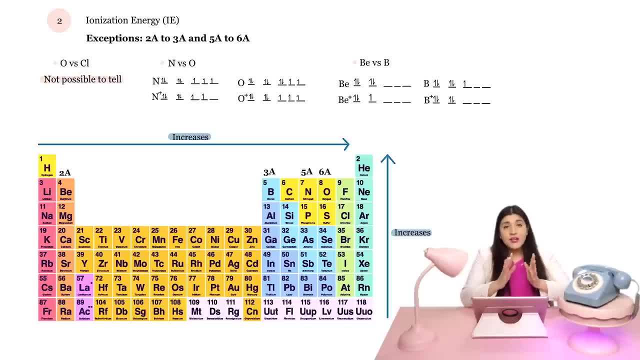 I know this is a little bit extra, but I just want to explain what's happening with this exception and why it doesn't work. If I were to write out the electron configuration and look at how many electrons are basically in beryllium- well, I know that beryllium here- 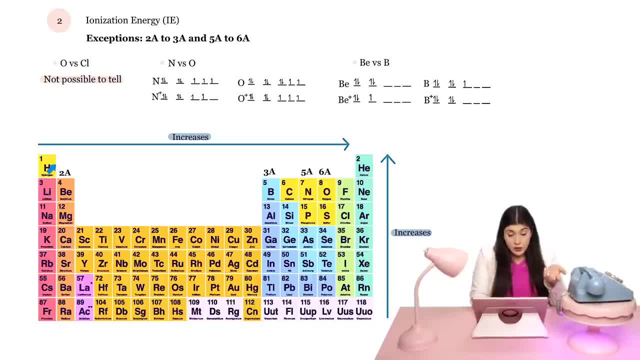 I start off with 1s2,, so 1, 2.. Here are two electrons in the 1s orbital, And then here I have 2s, right, So this is 2s, because this is 1, 2.. 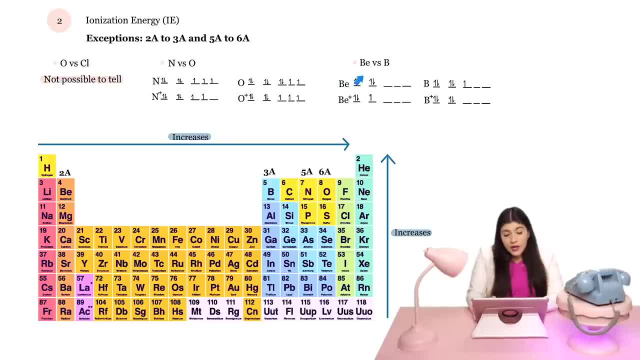 There are two more additional electrons, And this is a total of four electrons, since beryllium has four electrons. Well, if I'm removing an electron, then that means I'm removing one electron, Literally one electron, One of these electrons from this shell. 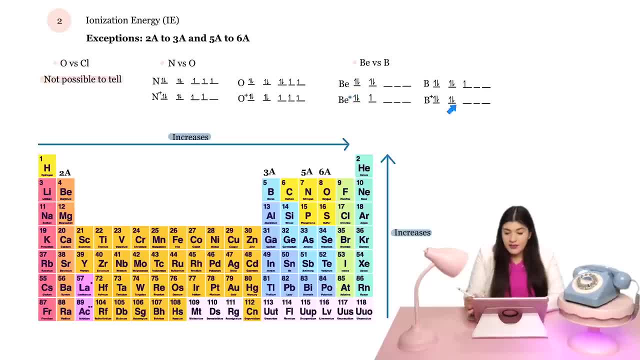 So this is what it would look like. And then now, if I'm looking at, let's say, boron, well, if I'm removing it from boron, now this is what we would have. So what I want you to necessarily think about is the opposite of what you're thinking essentially, with this exception. 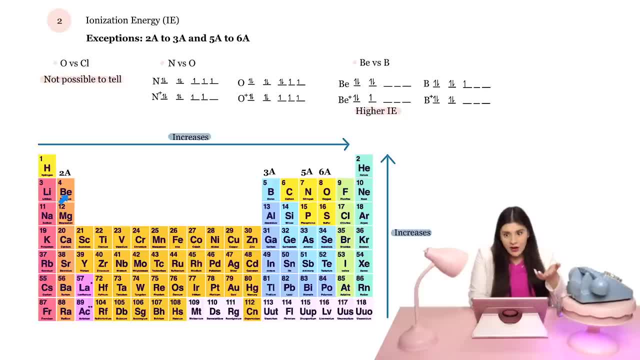 Where beryllium, though it shouldn't have a higher ionization energy, it does. So that's why 2A and 3A are going to be exceptions to this rule. The whole idea, and why I even showed this, was just looking at how much energy it takes to remove an electron. 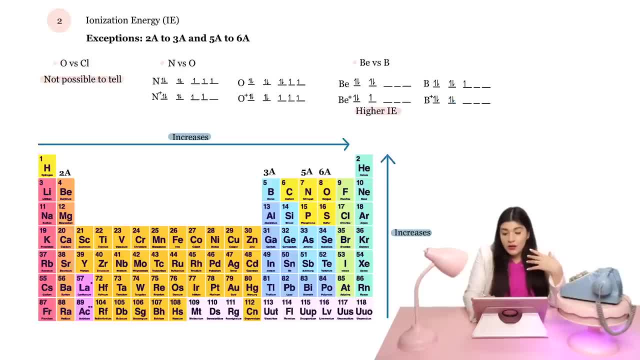 from something that's either half full or actually completely full. And what's half full? right, This is half full, this is completely full. So this would be a little bit harder to remove. So that's why it's explained by how many electrons we're removing. 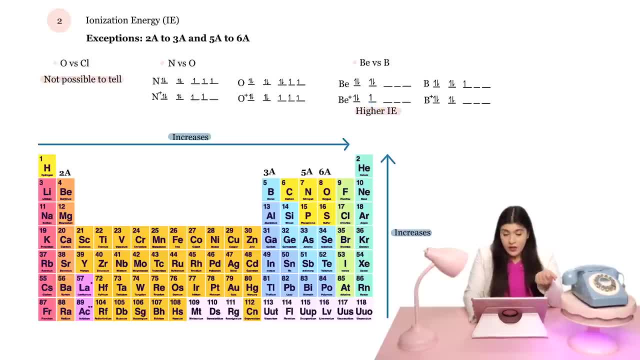 And essentially, if this is half full or completely full, Meaning this is stable and there's less energy there And this is not as stable, so there's higher ionization energy there. In this case, we know, going from 2A to 3A, that's the exception. 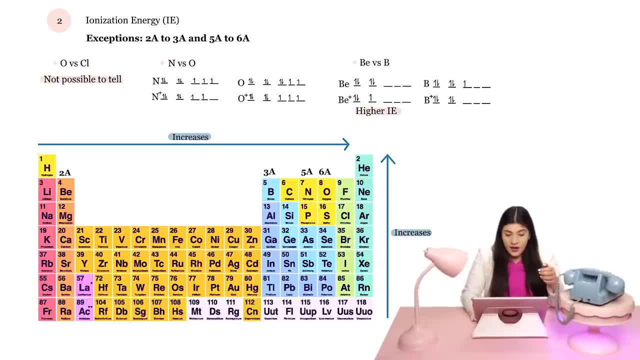 The other exception is, let's say, if we were going from picking atoms from 5A to 6A like nitrogen and oxygen. Well, once again, it's the opposite of what you're thinking: Instead of it being oxygen, it's actually going to be. 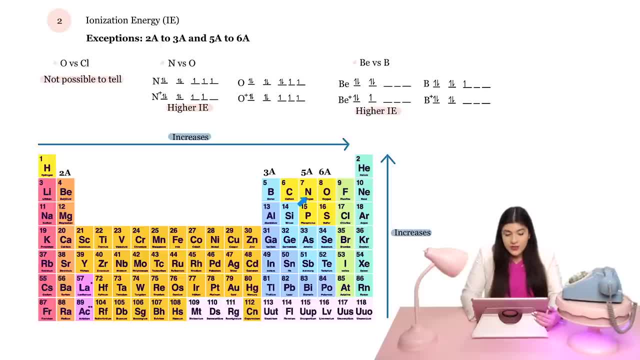 nitrogen that's going to have a higher ionization energy. So those are just exceptions to definitely know Anything that's equidistant from each other. there's not a way that we can determine whether or not something has a higher ionization energy. 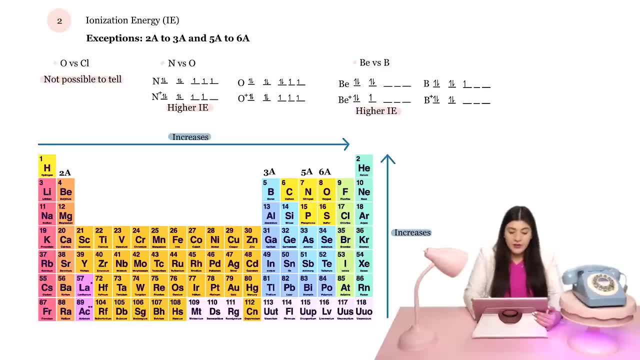 And whenever we have elements that are being compared from 2A to 3A, it's actually the ones in 2A that have higher ionization energies. And then same with 5A and 6A: the ones in 5A have a higher ionization energy than the ones in 6A. 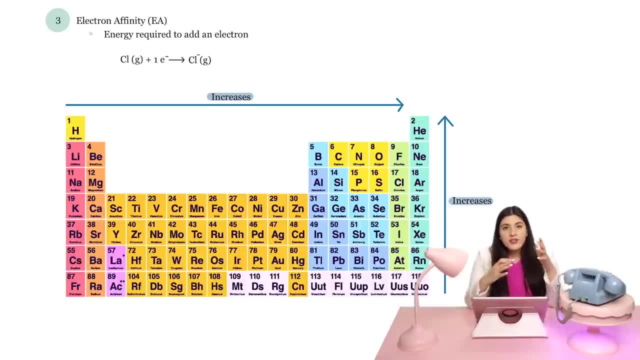 Moving on to electron affinity. So electron affinity is essentially kind of like the opposite of ionization energy. Remember, ionization energy was how much energy is required to remove an electron. Electron affinity is how much energy is required to add an electron. So we're doing this a little bit differently now. 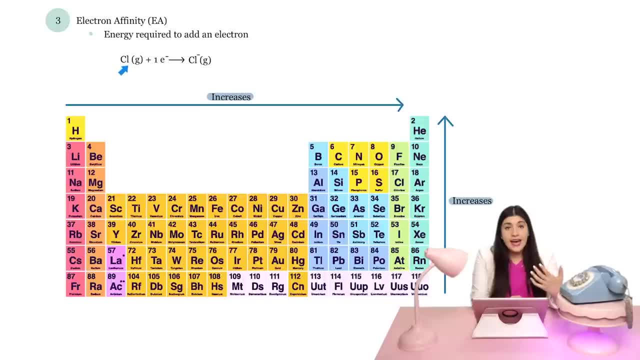 where, in this case, we're still going to have something that's in its gas form. And now what we're doing is we're adding an electron. So if we add an electron, it makes it more negative, right? That makes our atom an anion, in this case. 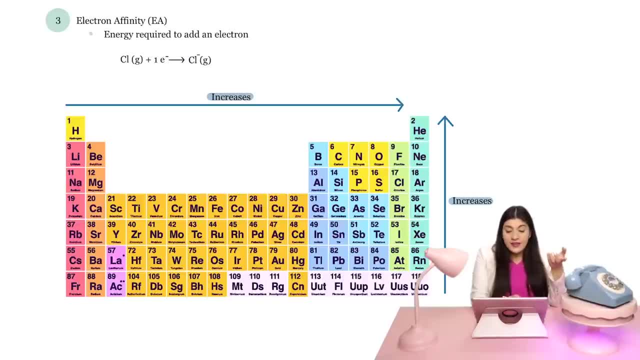 So a negative charge. So in this case, what I'm looking at again is the same exact trend really, where this is increasing as I get closer to fluorine, and this is increasing as I move up a column, So fluorine again is going to be a good way to remember this. 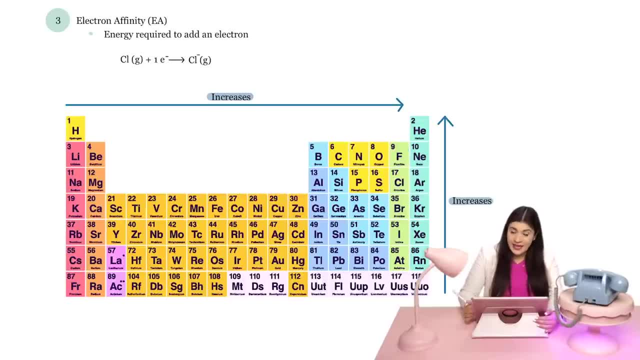 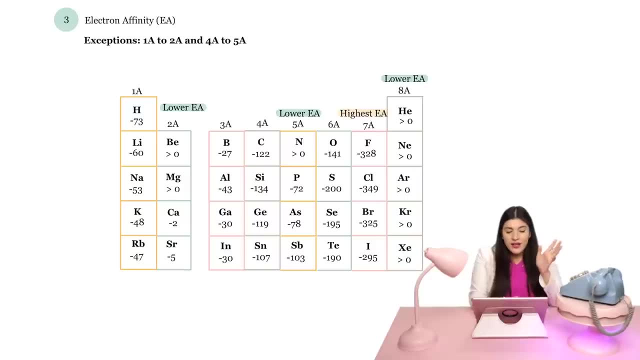 Whatever is closest to fluorine is going to have a higher electron affinity. Okay, so here are all of our exceptions, And I also went ahead and just wrote out how much electron affinity, like the actual numerical value, is compared to the most common ones that we have here on the periodic table. 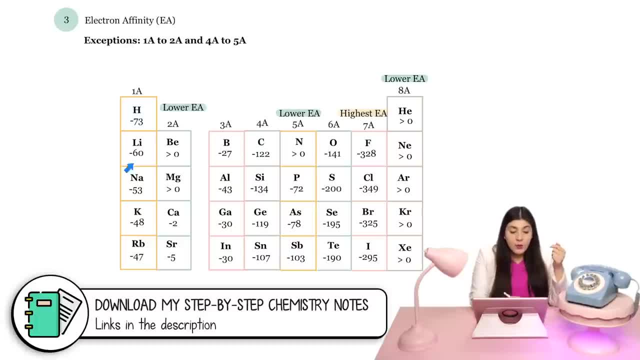 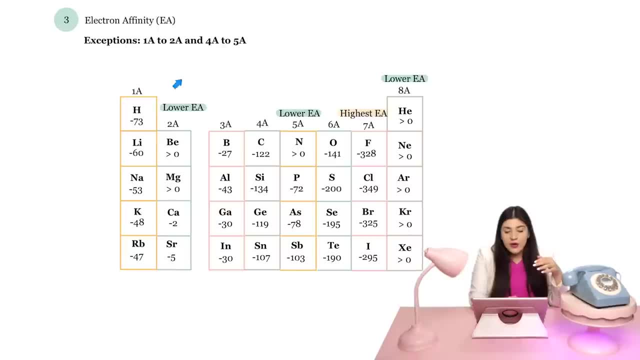 So your exceptions are going to be when we're going from 1a to 2a, And you'll notice that. sure, the trend said that we get higher in electron affinity if we're getting closer and closer to fluorine, or as we move across the periodic table. 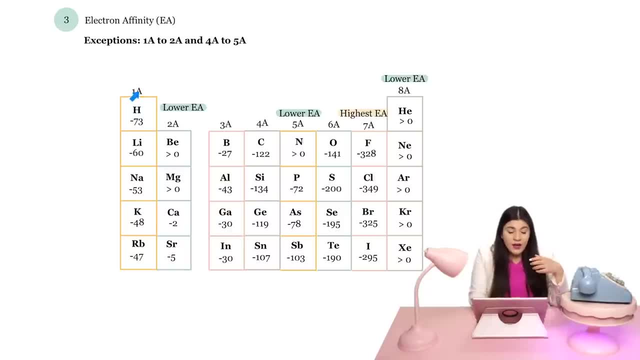 But that wouldn't be the case if we're comparing elements from 1a to 2a. So if I were comparing lithium and beryllium, beryllium actually has a lower electron affinity and lithium would have a higher electron affinity. 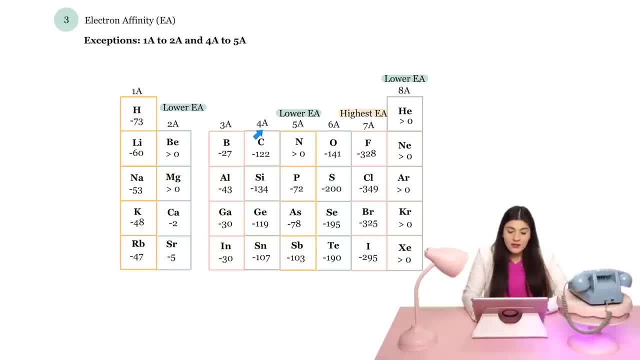 And then if I were to compare, let's say, something in 4a versus 5a, well, the ones in 5a actually have a lower electron affinity versus the one in 4a. So if I'm comparing carbon and nitrogen, 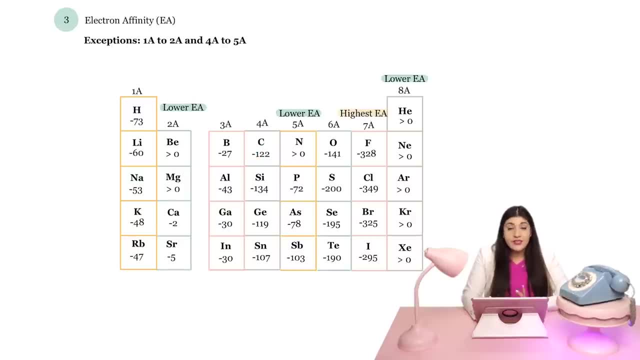 well, carbon has a higher electron affinity versus nitrogen, And the ones that have the absolute highest electron affinity are going to be your halogens. Something else to note is the noble gases will not have a high electron affinity. They're actually going to have a lower electron affinity. 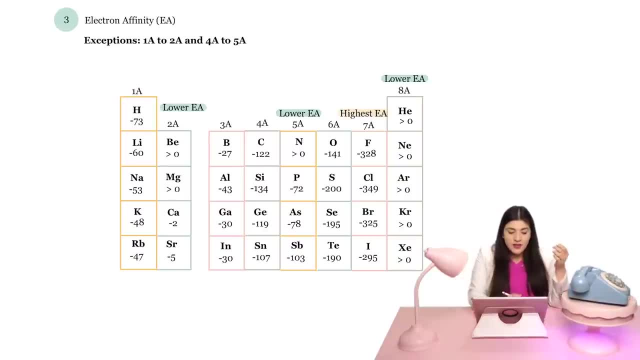 And I know this is kind of like counterintuitive, because electron affinity here is negative. Well, remember, if we're adding electrons we want it to be negative, right The more. if we keep adding electrons it means it's going to be a larger negative value. 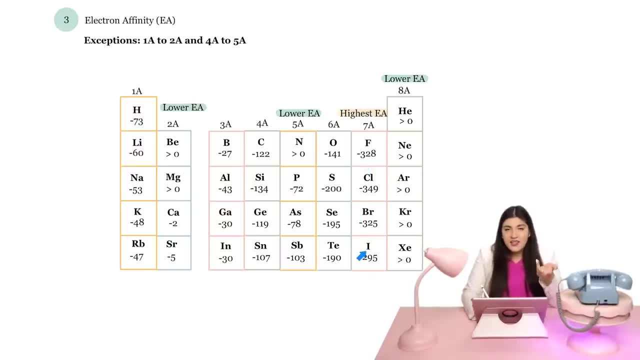 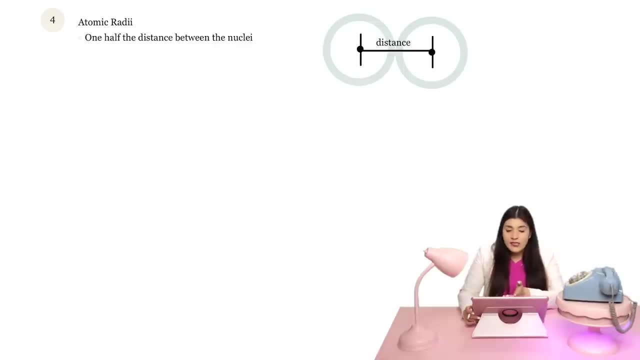 And the larger negative value tells us that that's actually a high electron affinity. Now, moving on to atomic radii. So what atomic radii is talking about is, let's say, if we were to have some sort of diagram like this, where this is representing one atom and this is representing a second atom of the same kind. okay, 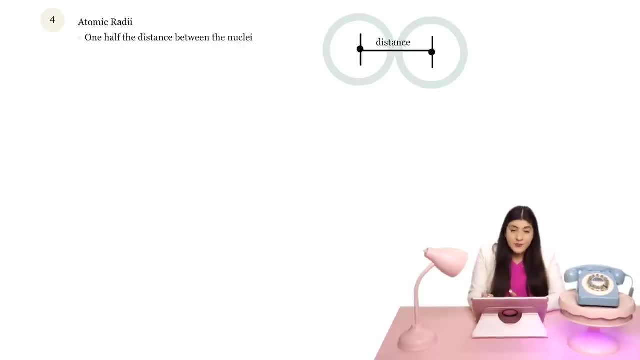 So let's say this is boron and boron or calcium and calcium. Well, what we're measuring for atomic radii is it's the distance between the radii, And we take half of that, So it's divided by 2.. 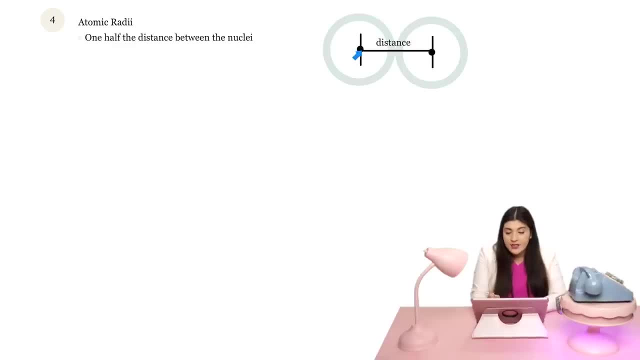 So it's one half the distance between the nuclei right. This is the nucleus, This is the nucleus. These together are nuclei. So it's this distance is what we're essentially measuring, And we're seeing which one is larger, which one is smaller. 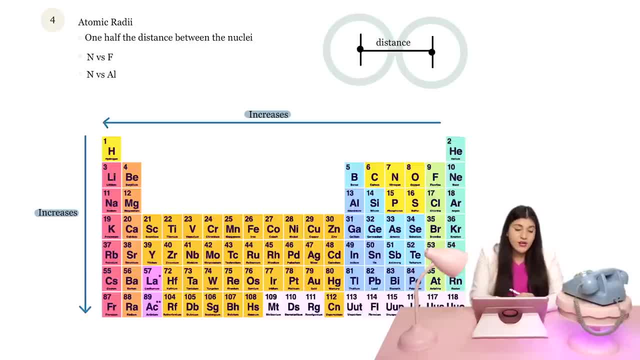 So we'll do those examples in a second, And then this is our trend. So our trend has changed. It's the complete opposite, where before, with everything that we were seeing, electronegativity, ionization, energy and electron affinity was in this corner right. 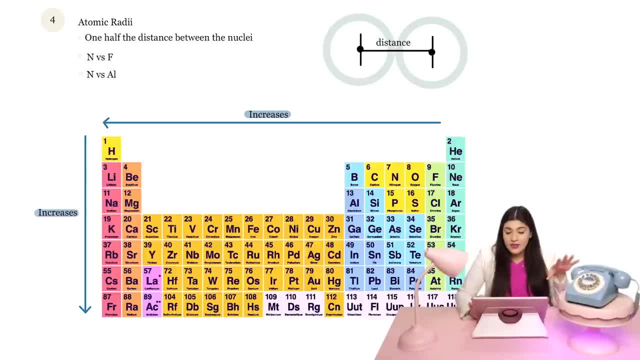 Fluorine was pretty much the highest in all of those, And now it's the complete opposite. We're looking at this corner, Whatever is closest to CS or FR or radium or you know, this corner overall that's going to have a higher atomic radii. 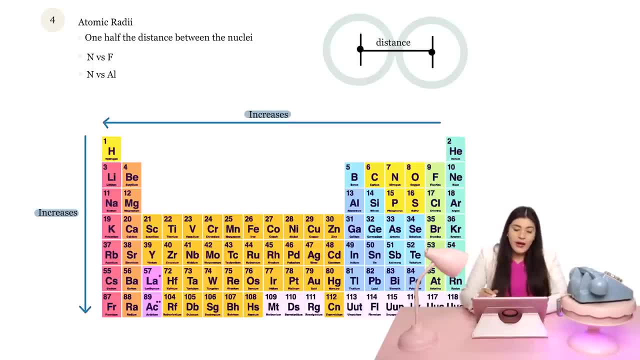 So it increases as we go the opposite way, as we go from right to left on our periodic table and then as we move down a column. So now let's actually attempt this and let's look at nitrogen versus fluorine. So nitrogen is here and fluorine is here. 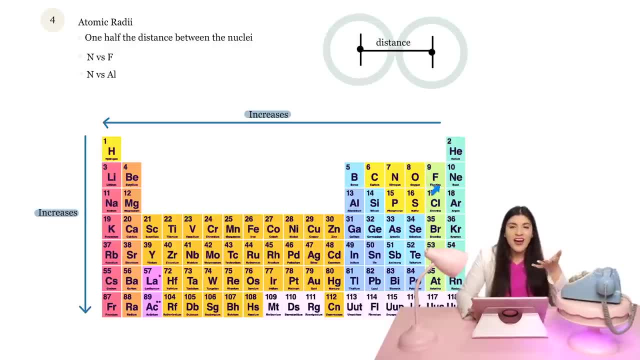 So fluorine no longer has the highest atomic radii, or it's no longer the highest in something. In this case, for atomic radii, it's actually lower. So nitrogen would have been the one that has a larger atomic radii. And then now, if we're comparing nitrogen and aluminum, 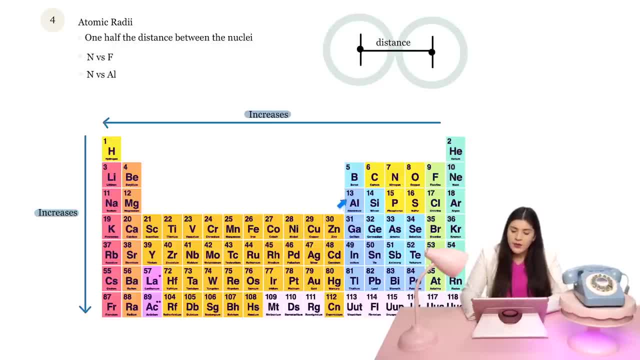 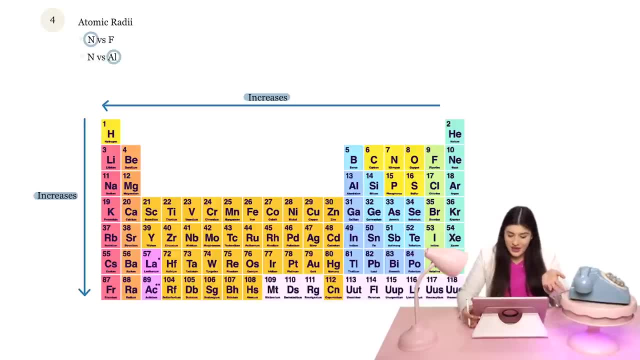 well, aluminum is a little bit lower on our periodic table, So I know that aluminum is now going to be the one that has a larger atomic radii, And then those are just the answers there. Okay, So this still has something to do with atomic radii. 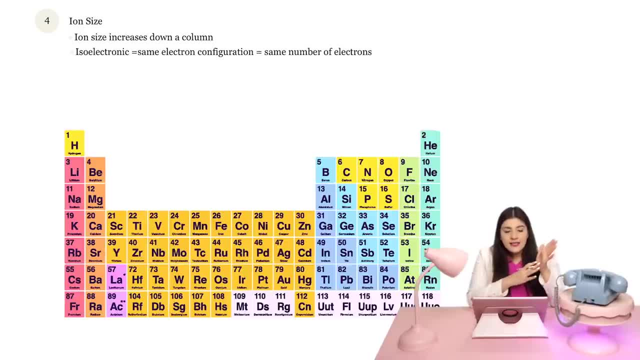 It's just a little bit different now. So instead of looking at something that is neutral, we're going to talk about an ion. So this is ion size. Remember what an ion is. An ion is simply an element with a charge. Okay. 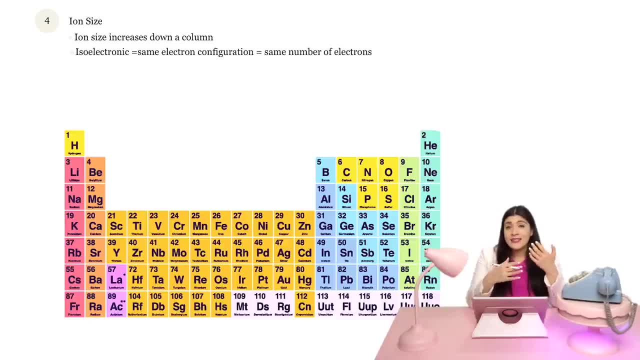 So you could either have something that's an anion, meaning the element has a negative charge, or you can have a cation. Cation just means the element has a positive charge. So what's essentially happening with this, this ion size? 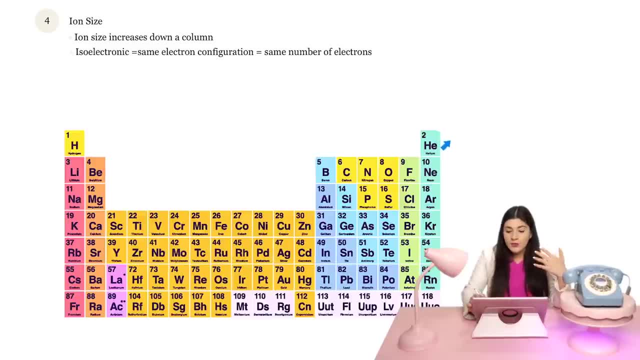 is that it increases as we go, As we move down a column. So as we move down a column, Now it's not as simple as the other trends, I'd say. You do have to look at a lot of different factors, which we will go over. 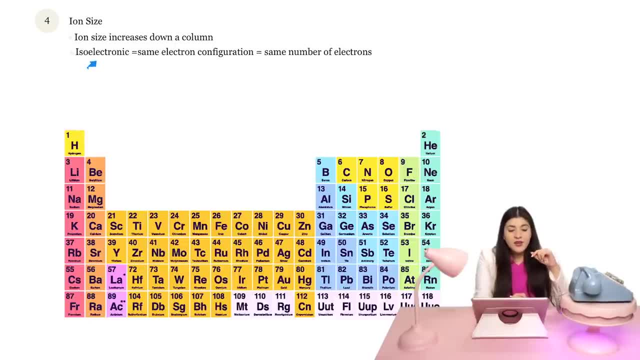 There is something else that I definitely want you to know. This word, isoelectronic, just refers to there being the same amount of electrons, And if there's the same amount of electrons with the elements, like, let's say, if we're comparing two different elements. 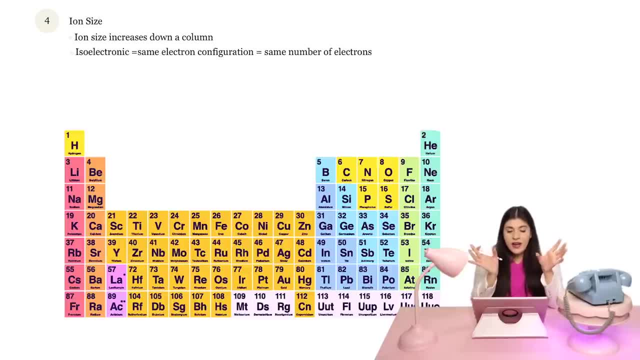 and one has a charge and another one doesn't, and we find that they have the exact same amount of electrons, then we would say that this is isoelectronic, because they have the same amount of electrons. You could also see that this would have the same exact electron configuration. 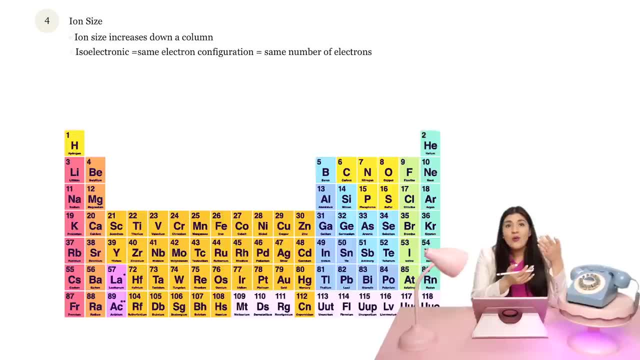 because with electron configuration, we're essentially seeing where are these electrons going, what orbitals are they going in and how many electrons we have. So let's say, if we're trying to compare all of these, okay. So if I were to try to compare, let's start off with sulfur. 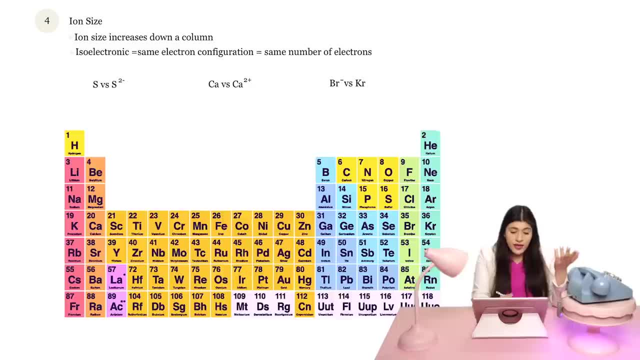 and this anion of sulfur. Well, the first thing I want to do is just count up the number of electrons and compare it that way. okay, So I'm going to start off with just identifying how many electrons I have. So how I'm going to do that is by looking at my periodic table. 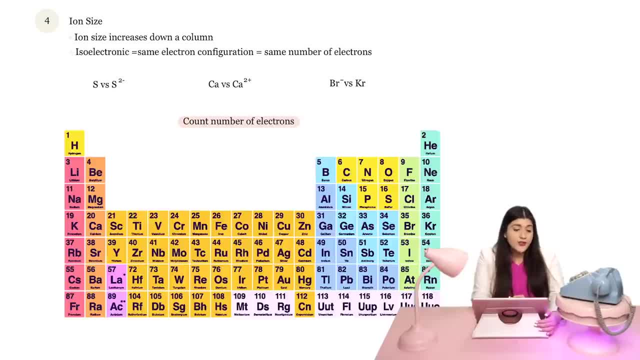 I'm going to look at the atomic number, And because sulfur here is neutral, then the atomic number is going to tell me exactly how many electrons there are, so 16.. So I know, okay, there's 16 electrons for sulfur. 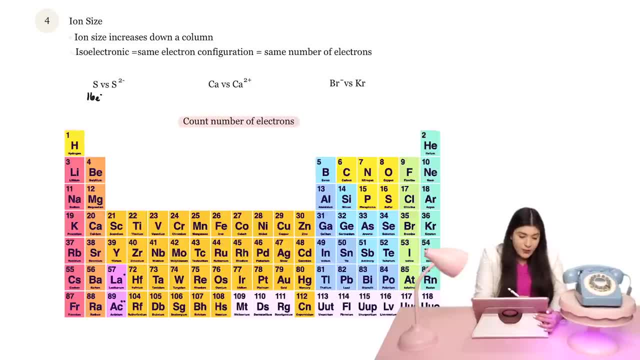 Now, if I'm looking at sulfur with a 2- charge, well, remember what this 2- means. This 2- actually means that we're going to add electrons. okay, because electrons are negatively charged. So this would have been 16 plus 2, giving us 18 electrons. 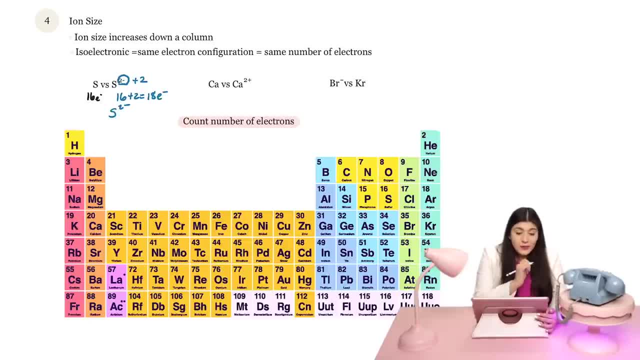 So the anion is going to be the one that has the larger size in this case. Now, let's say, I'm comparing calcium versus calcium 2+, So now we have calcium in its neutral state and then the other one is going to be the cation. 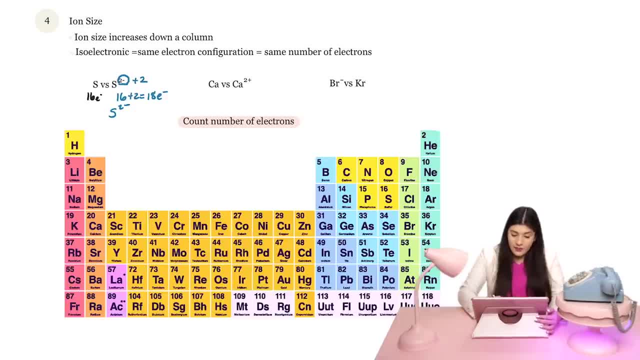 So with calcium, I know let's look at the periodic table again. So calcium is here and I see that that's 20, so calcium has 20 electrons. So, okay, 20 electrons. Now, since this is a 2+, this is the opposite, okay. 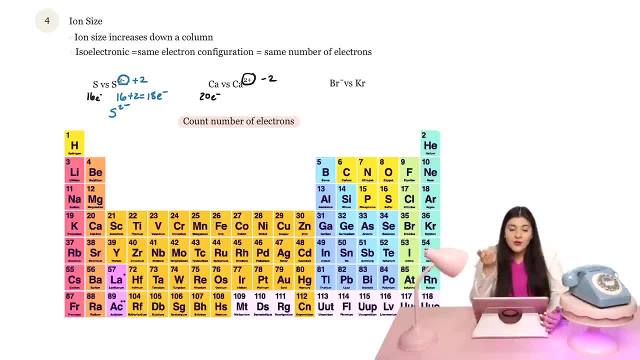 We're actually subtracting 2 electrons from 20, the initial amount that calcium has. So 20 minus 2 would then give us 18 electrons, And I see, okay, which one has more electrons? Well, the one that has 20.. 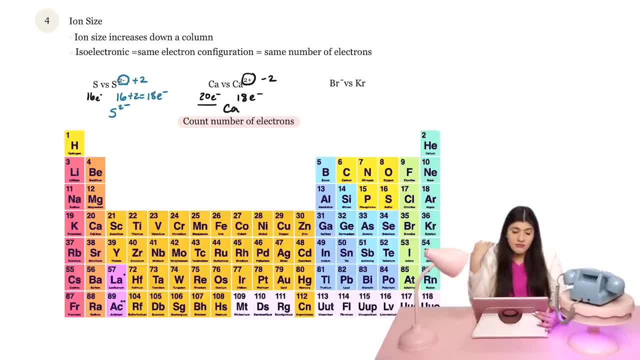 So calcium in its neutral state is then going to be the one that has the highest ion size. Now, if I'm comparing these two different ones, okay, so I'm going to start off with just the noble gas of krypton and figure out the electrons. 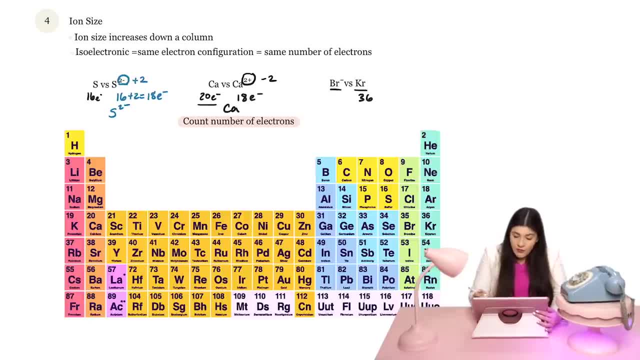 So there's 36.. And then now I'm going to look at bromine. So, starting off with bromine, that's here. There's 35. However, there's one electron here. okay, If it doesn't tell you how many. 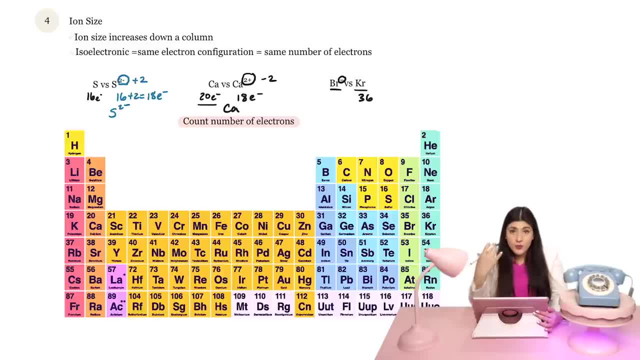 and there's just a negative sign or a positive sign, assume that it's just one. So what I have to do with 35 is I have to add So 35 plus 1, that also gives us 36 electrons, And notice that both of these have the exact same number of electrons. 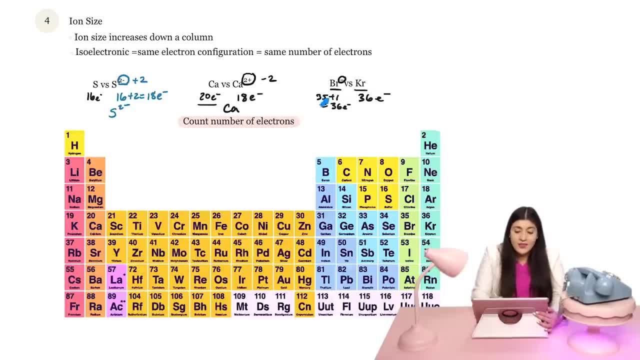 meaning they are isoelectronic. So these would be referred to as isoelectronic, meaning we don't necessarily know which one has the larger ion size. but if we really had to tell so we could state that this is isoelectronic. 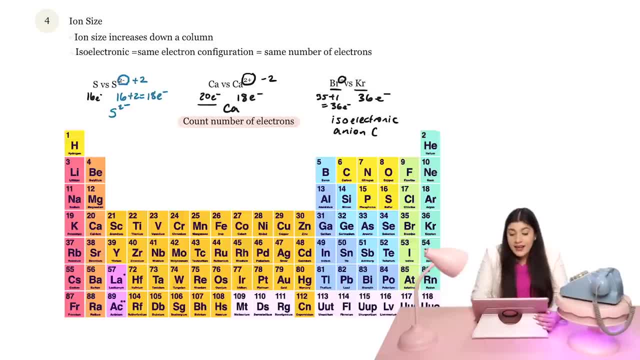 but if you needed to keep going with this, the one that has the anion or the negative charge is going to be the highest in ions, And there's a little chart for this that I made to help you be able to identify. okay, how do I know if anions are larger or cations are larger? 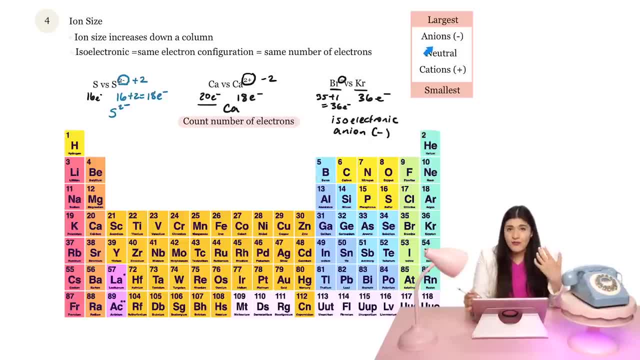 Anions are typically always going to be larger. okay, That's what we start off with. So anions are going to have the highest ion size. Then, following that, are going to be the ones that are neutral, the ones that have no charge. 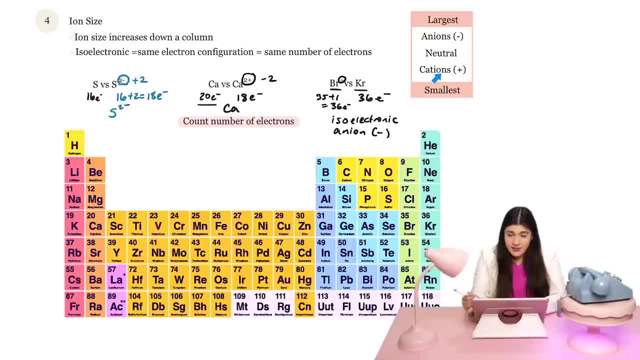 Then, at the very bottom, the smallest ion size are going to be our cations, okay. So that's definitely something to know and that's what we saw here, where, in this case, okay, we have neutral versus anion, and anion was the one that was, you know. 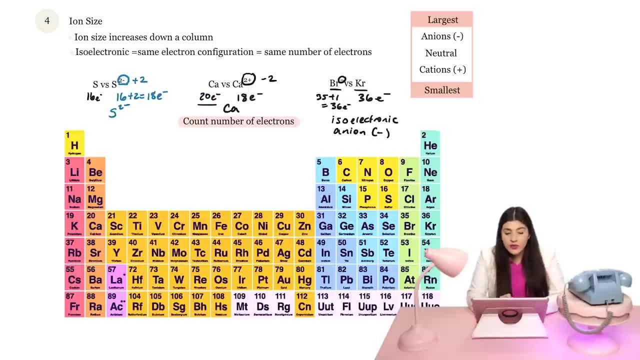 the highest ion size. Here we have neutral versus cation. well, neutral is higher. And then here, if we're comparing something that's neutral and anion, then I know that an anion is going to be the one that also wins in this case. 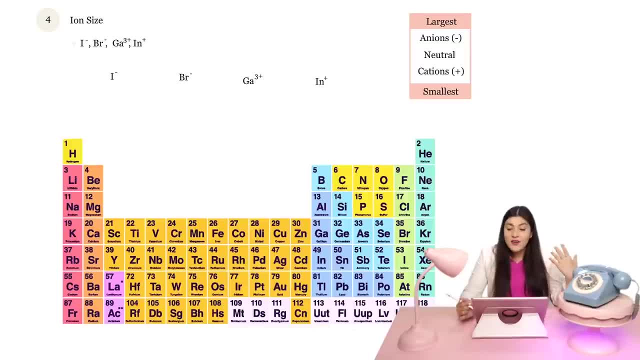 and it's the highest ion size. Let's do another one of these where let's say if we have a bunch of them, we have a bunch of different ones and we're trying to see which one. let's say, if we're doing this in from lowest to highest, 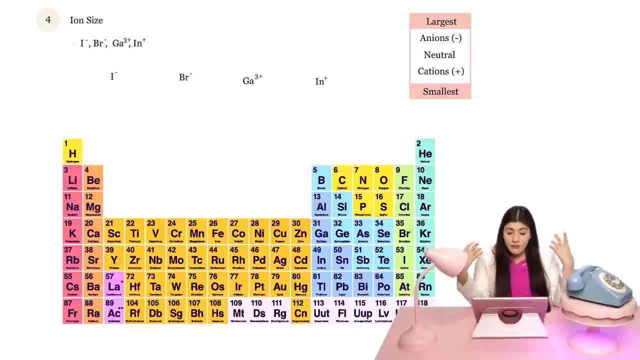 or increasing order. well, what I want to start off with is just identifying how many electrons we have for everything. okay, Let's do this together- and I did this already, but let's do this together still. Let's say, for iodine, that's 53.. 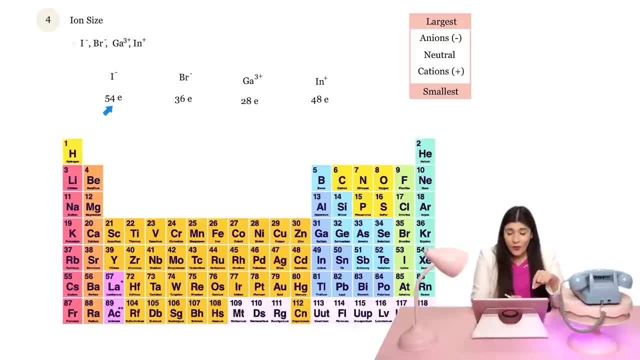 So 53 plus this additional one here, that's 54.. And then next, for bromine, we said: okay, well, there's 35 plus this additional electron, so that's 36.. For gallium, we have that's here, so that's 31.. 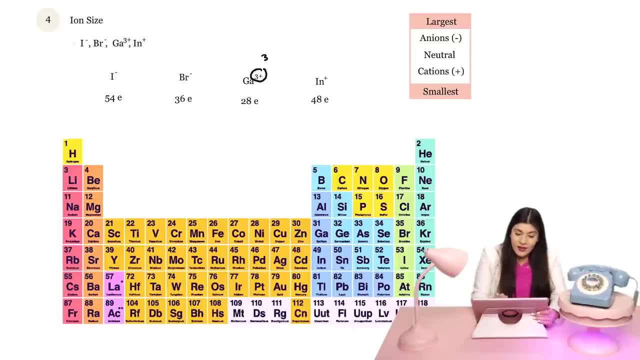 But I am subtracting three from 31.. So 31 minus three, that's where I get that 28.. And then next for IN, that is here That's going to be 49 minus one, because I'm subtracting that one. 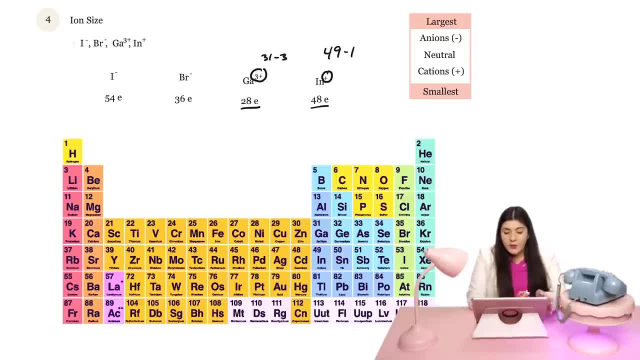 So that's where I get that 48.. You would think that okay, because we have all of this, I can just order this from the lowest amount of electrons to the largest amount of electrons, but that's not the case here. This still applies, okay. 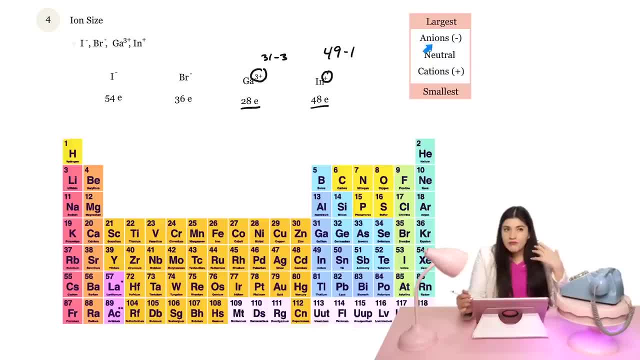 Where our anion is going to be first. right, It's going to be the largest. This is what we would actually see. We're going to look at both of these first. okay, And I'm not, I don't even care about IN right now. 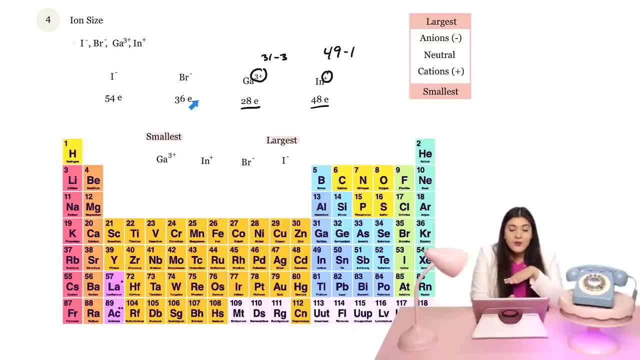 even if that has 48 electrons. Right now I'm just comparing the two different sizes of the two different anions that I currently have, Because they have the same charge, because they're both one minus and one minus. I know the next, the deciding factor or the tiebreaker. 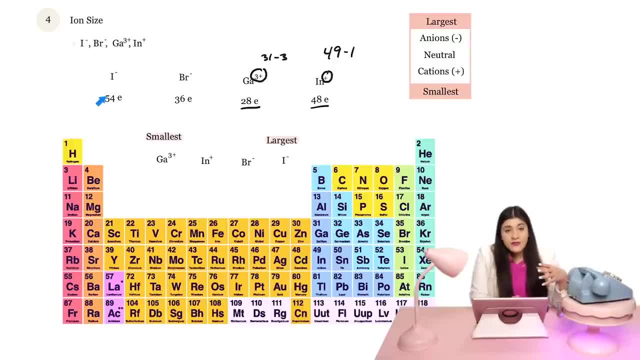 is to look at the amount of electrons. So here this is 54. So because it has a larger amount than the 36,, then I know that that has to be the largest. The one that follows is then bromine, not IN. 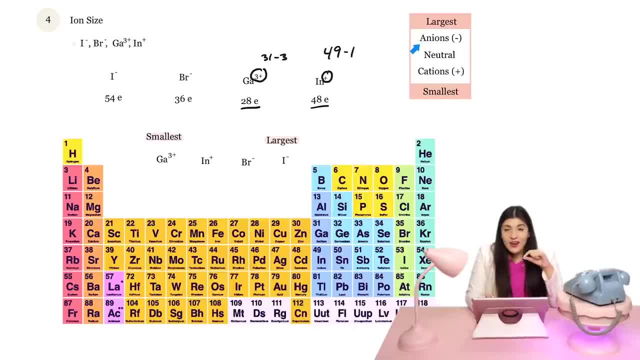 And the reason for that is because anions are the ones that have the largest ion size. Then after that I look at my cations, since there's nothing that's neutral. But if there was something that was neutral, that would go next. 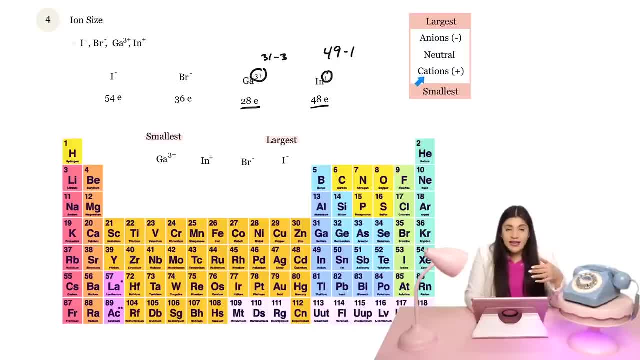 But because there's nothing that's neutral. I now look at cations and I see well which one has one, the lowest cation, which is one in this case. And if this were the same, if both of these had like plus one plus one? 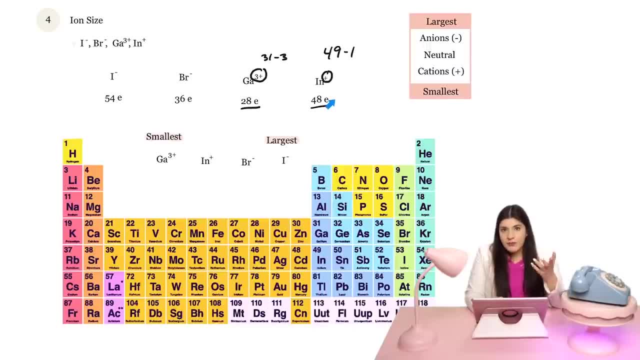 then I would go and look at the electrons and that would be my tiebreaker again. So this is what comes next, And because this has the highest positive charge, or this is the largest cation, I know that that's actually the smallest ion size. 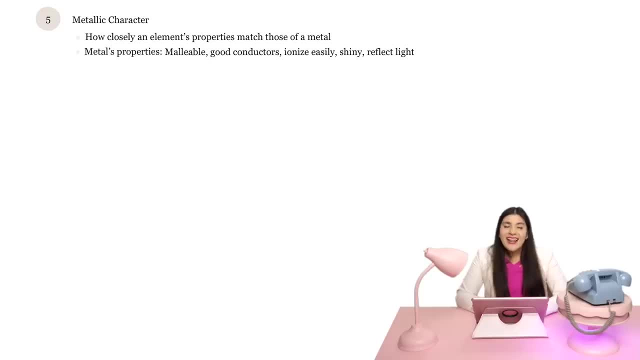 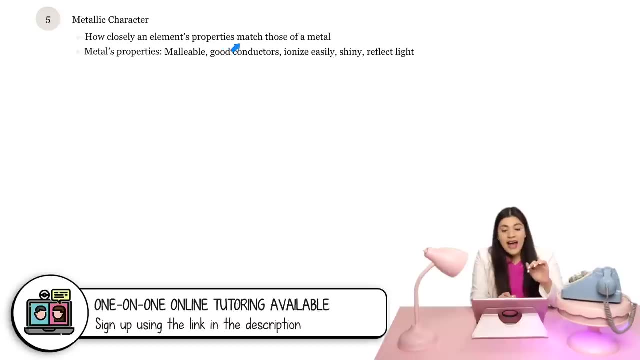 Okay, so that's how we would rearrange this for ion size. There's one more Metallic character. So when we're talking about metallic characters, we're essentially looking at how closely an element's properties match those of a metal. So we're looking at what is a metal. 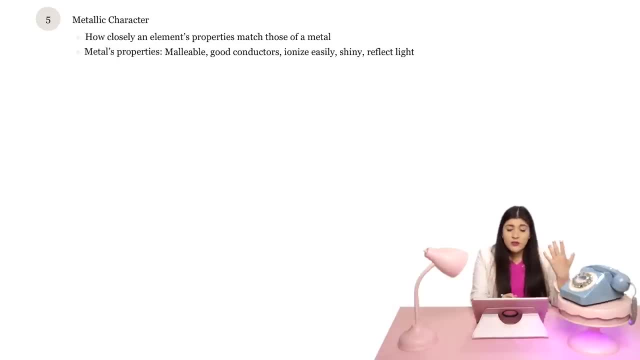 You know what are the properties of a metal. So a good metal, or a metal overall, is going to be malleable. It's going to be a good conductor, so a good conductor of electricity. typically It'll ionize easily. It's shiny. 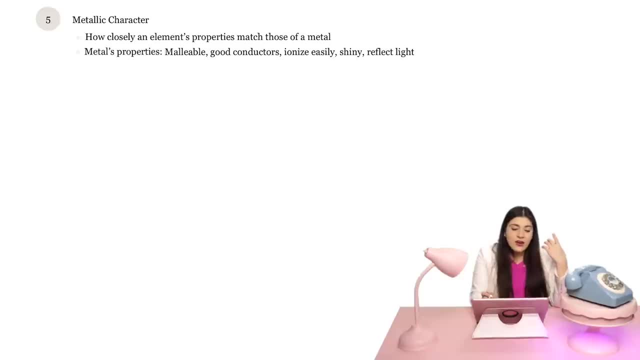 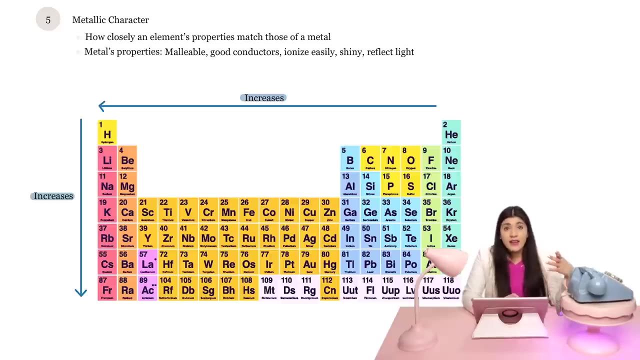 It's going to reflect light. So all of these different things are properties of a metal. Now, this is the overall trend. So this actually is very similar to atomic radii, that trend where everything in this like bottom corner or as we get you know closer here, 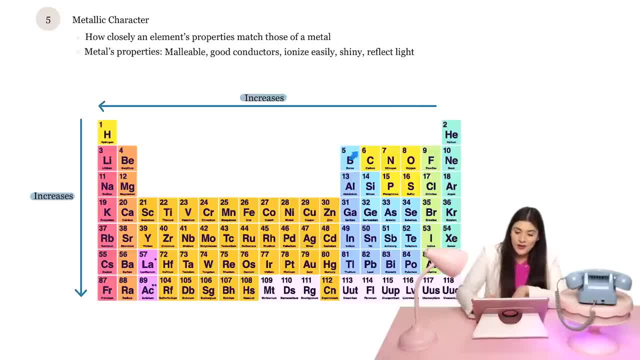 I'd say moving away from the noble gases and all the nonmetals. right, These are all of our nonmetals, which makes sense why those wouldn't have metallic character. It's everything here which remember our periodic table. Well, these are our transition metals. 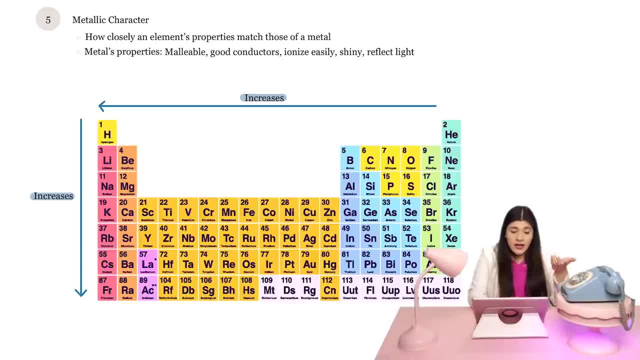 and these are two different types of metals as well- right, Our alkali metals and our alkaline earth metals. So that's why the trend is moving in this direction And away from the nonmetals, because these would have the most metallic character. 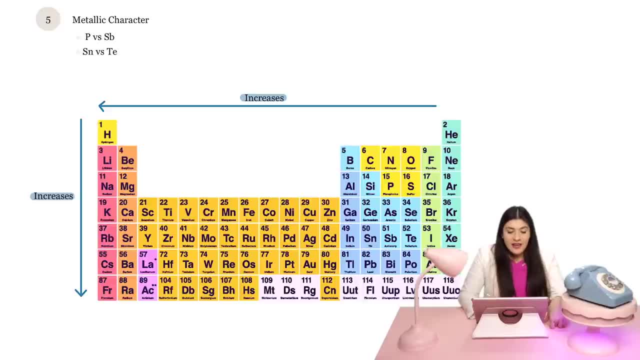 just meaning they would behave more like a metal. And then here let's actually do some. So I'm comparing phosphorus and what is this Sb? So let's find that, Let's find that. So Sb's here. 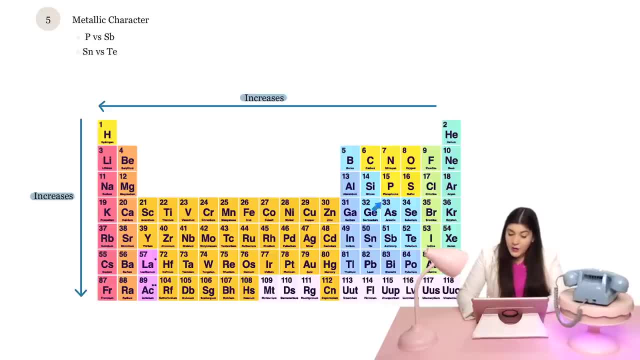 So we have Sb and then we have P, your phosphorus. So if I'm comparing both of these, they're in the exact same column. So I see, okay, well, because this is lower, that must be the answer here. 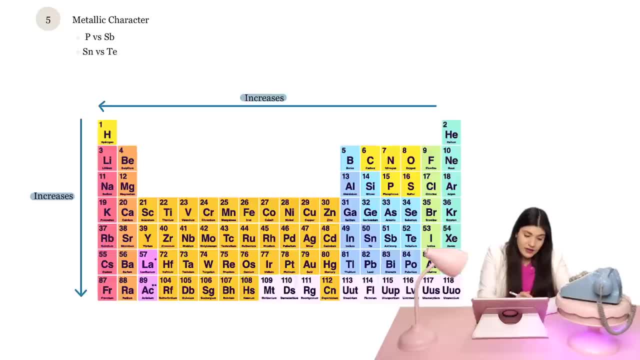 That has to be the case where this is. this is going to be our answer: That's going to behave more as a metal. And then now, if I'm comparing Sn and Te- so Tin, which is here- then I'm comparing both of these actually. 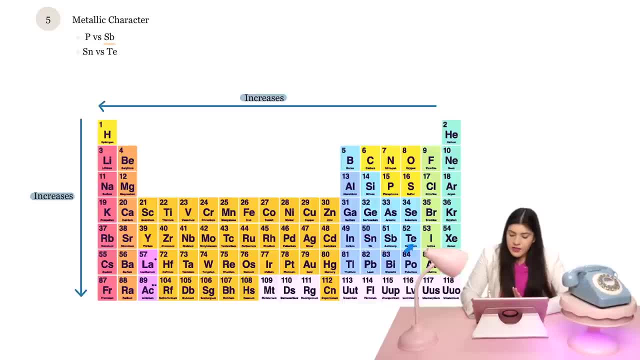 Sn and Te. Well, if I'm comparing both of these, which one is more to the left of my periodic table? that's going to be Tin. So Tin, So Tin would have been our answer in this case. So those are the answers that we have overall circled. 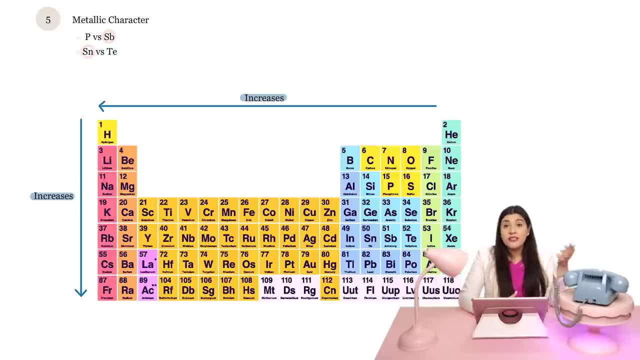 And that's how you would actually define all of these and understanding all of these periodic trends. Definitely know your periodic trends and this will come up again just to let you know, especially electronegativity, If you're going to learn any of these. 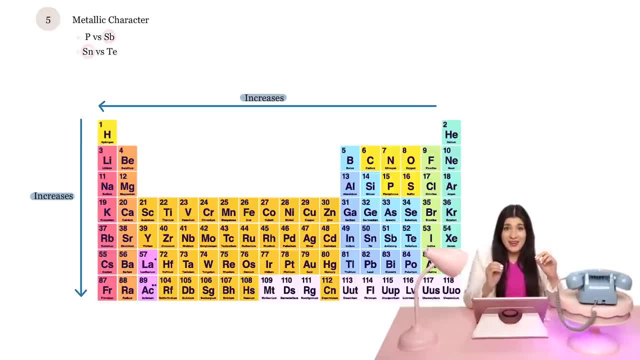 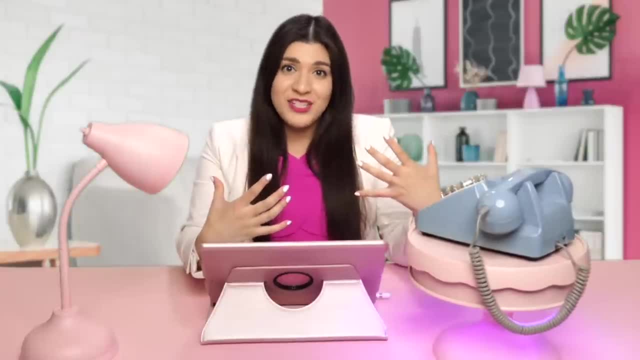 which I want you to learn. all of them know electronegativity, okay, Now if you want to get your question answered- because I know you got a question or you will eventually have one- then check the description box. There you're going to find the link. 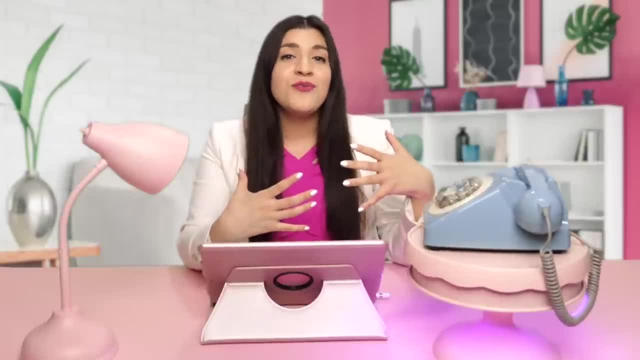 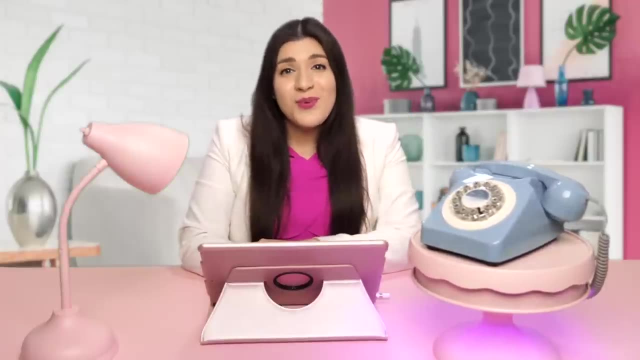 and it's going to take you to a form that you'll fill out and you could ask your question and I'm happy to answer it. Since you're in the description box already, then make sure to check out all of the other resources. 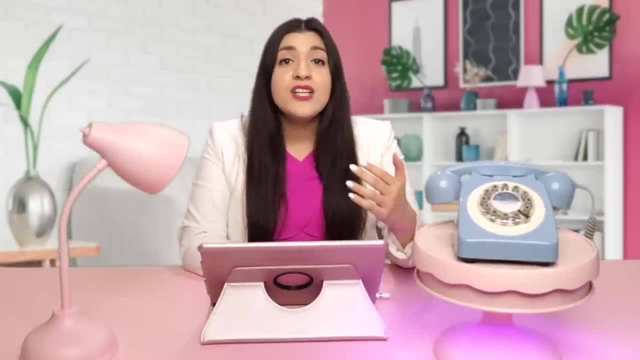 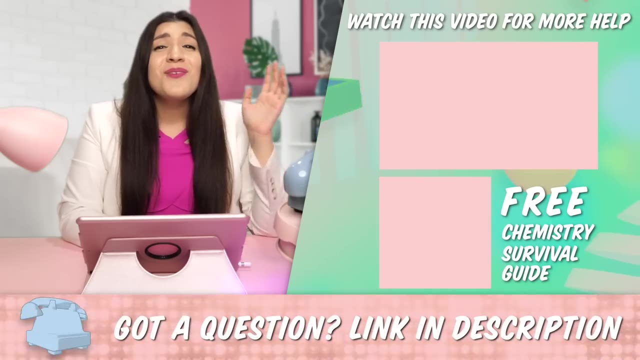 that I know can help you pass chemistry, because I don't want you to retake this class and I know you don't want to have to do this over again. So look at all of the different resources that I have and I'll see you in the next video.